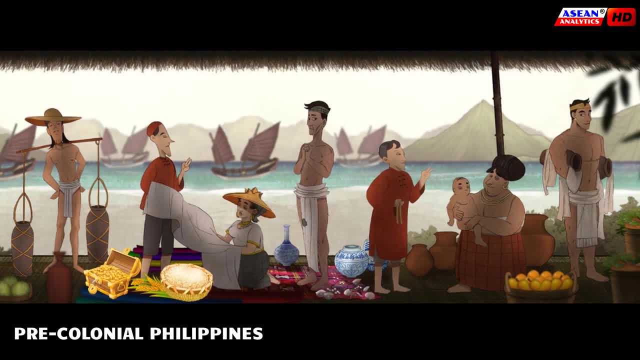 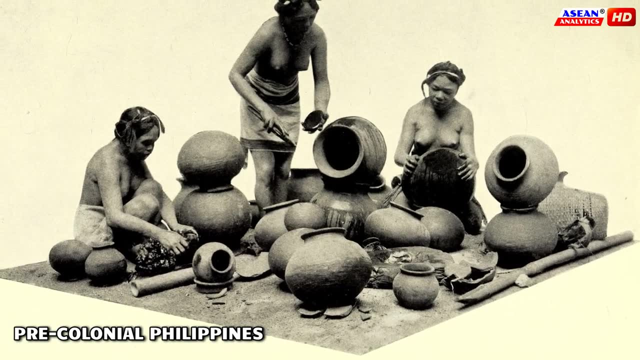 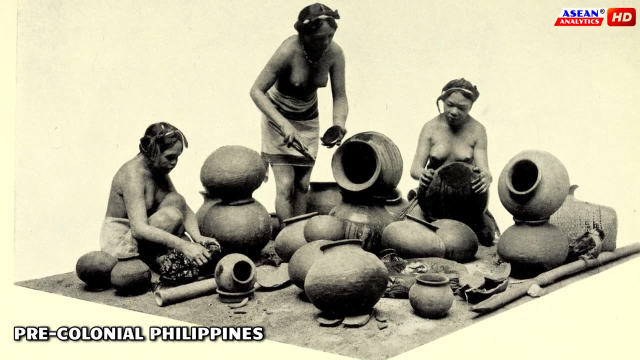 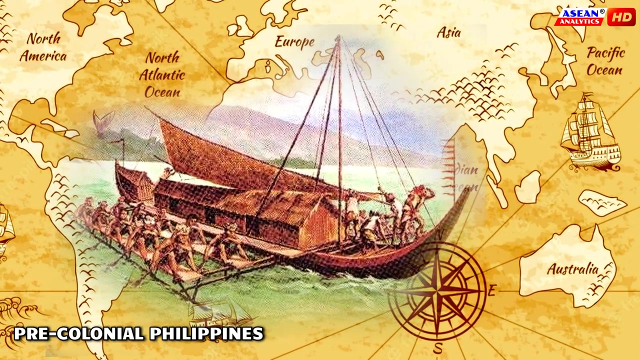 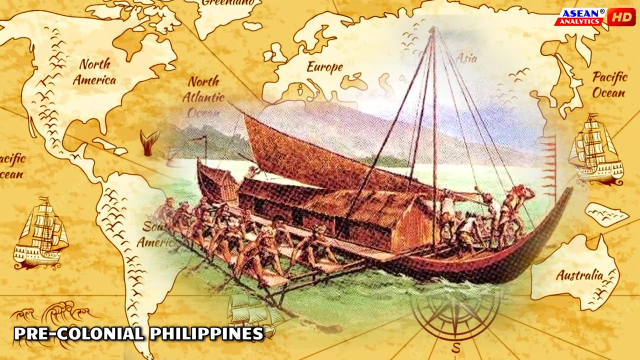 hostage exchange or outright raiding from Filipino kingdoms was also present during those ancient times. From the 12th century, the Philippines' economic history has been traced back to the 11th century and the 18th century 18.. The American community in the Philippines' economic history hasjoined the world's leading dichotomy From the 20th century. the American community in the Philippines' economic history has been traced back to the 11th century and the American community in the Indian community hasjoined the world's leading dichotomy: The top-uclar based trade in the Philippines in the 15th century was the Sochi, Kangam, Magadan and Tauang. In the 15th century, the Philippine people were most active in international trade and they used the ocean as a natural highway. Ancient peoples were engaged in long-range trading with their Asian neighbors as far as west as Maldives. 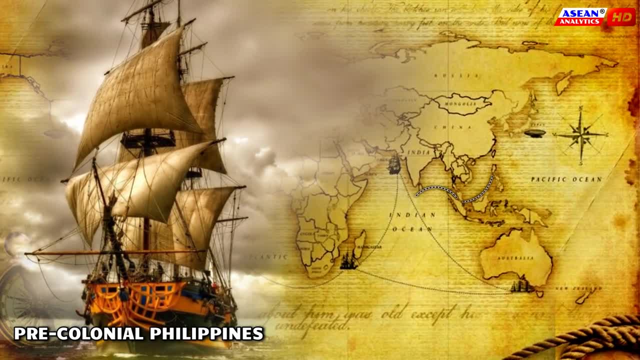 and as far as north as Japan. In the Western period, the Arabic and Chinese were replicate in the of the Philippines. particularly, Manila was part of the maritime hub in Southeast Asia, together with Malacca, connecting the Indian Ocean through the Strait of Malacca to the South China Sea. 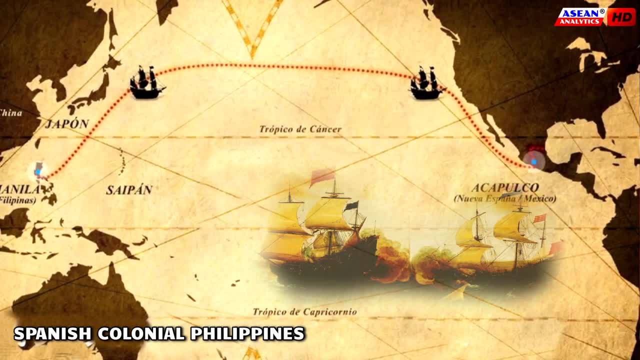 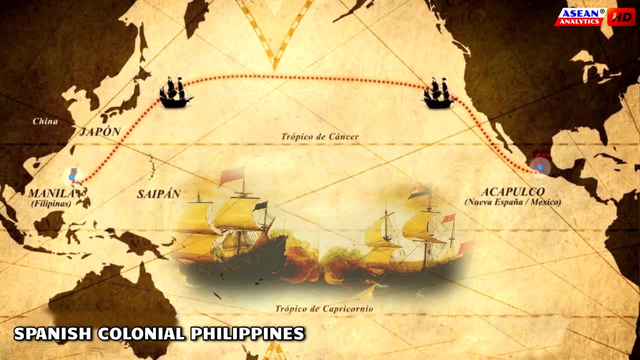 During the Spanish colonial period, the economy of the Philippine island grew further when the Spanish government inaugurated the Manila Galleon trade system, Where trading ships, settlers and military reinforcements made voyages once or twice per year across the Pacific Ocean from the 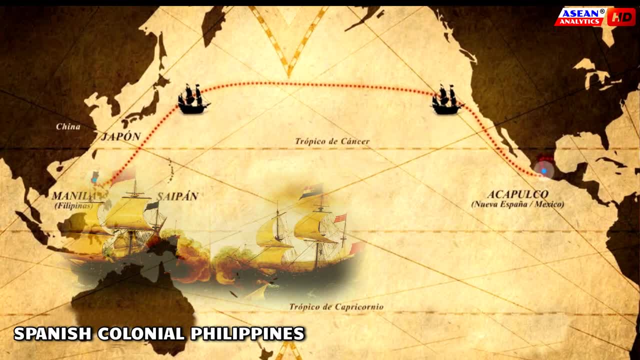 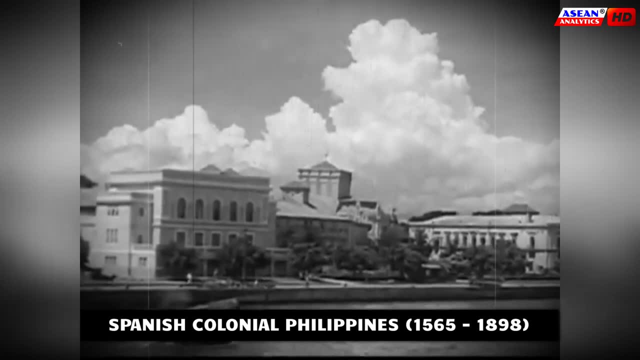 port of Acapulco in Mexico to Manila in the Philippines. This trade made the city of Manila one of the major global cities in the world. The Philippines also became the distribution center of silver mined in the Americas, which was in high demand in AsiaDuring the period, the country 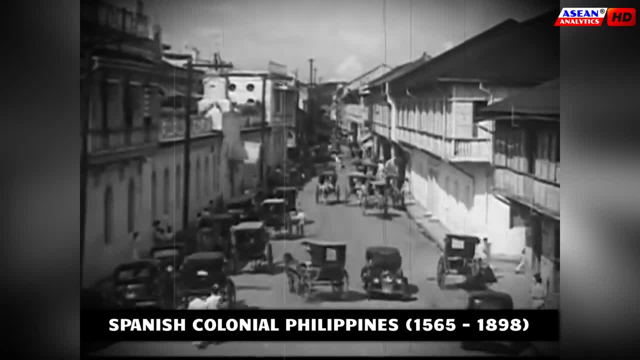 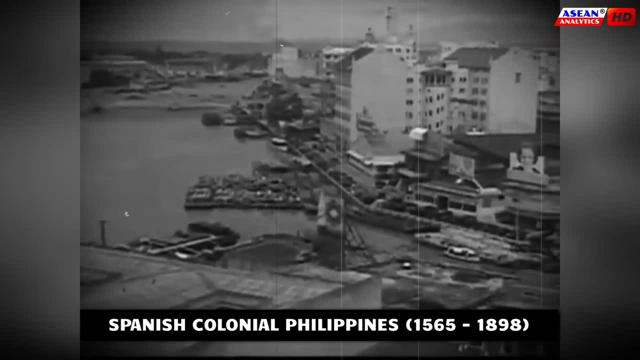 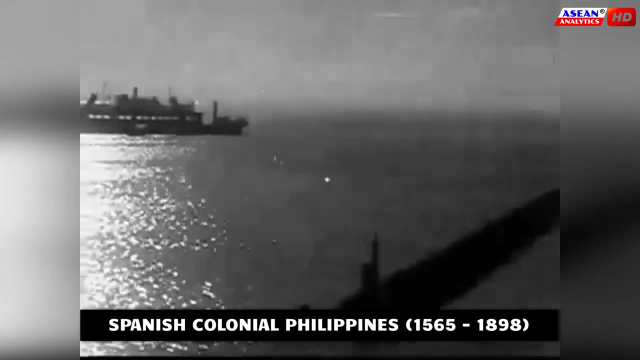 was a trade entrepot between the nations of South East and Southeast Asia and the territories in Spanish North and South Americas. Various manufactured goods imported from China, Indonesia, Malaysia and India were imported into the Philippines and were re-exported to Mexico or Peru. The Manila Galleon system operated until 1815, when 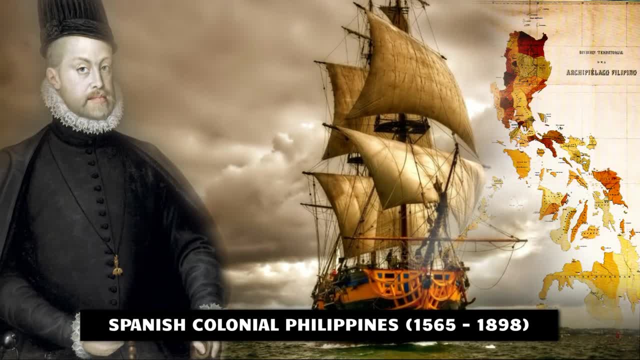 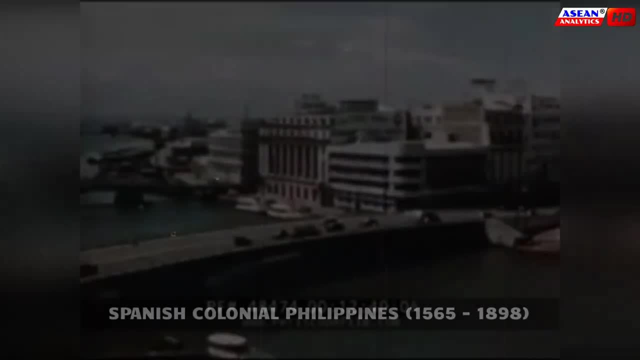 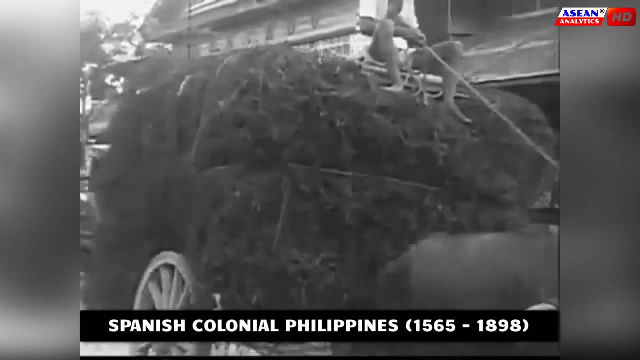 Mexico got its independence. This resulted in the Philippines being governed directly by the King of Spain and other Pacific islands to form the Spanish East Indies. It made the economy of the Philippines grow further as people saw the rise in opportunities. Agriculture remained the largest contributor to the economy, being the largest producer of coffee. in Asia as a whole. The Philippines' economy was the largest producer of coffee in Asia as a whole, as well as large production of tobacco. The economy of the Philippines rose rapidly and its local industries developed to satisfy the rising demands of an industrializing Europe. In 1834, the Royal 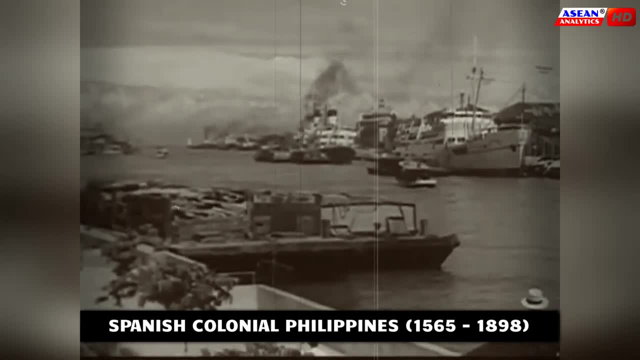 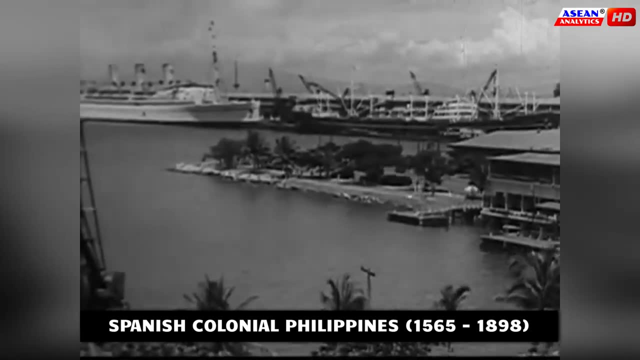 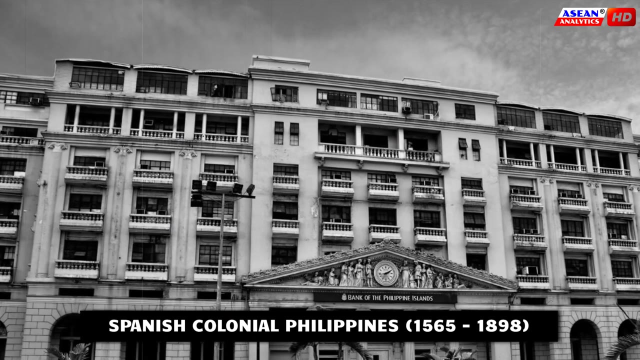 Company of the Philippines was abolished and free trade was formally recognized. With its excellent harbor, Manila became an open port for Asian, European and North American traders. European merchants, alongside the Chinese immigrants, opened stores selling goods from all parts of the world. The El Banco Español Filipino de Isabel II – now Bank of the Philippine Islands – was the. 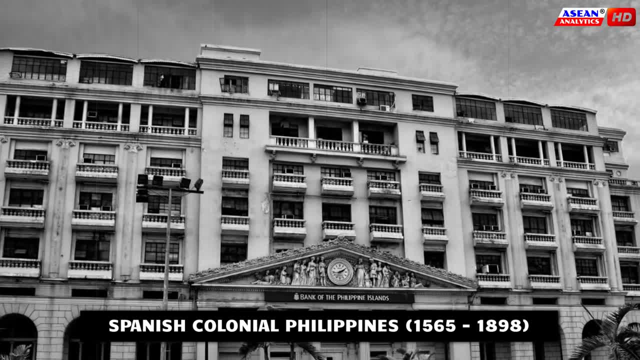 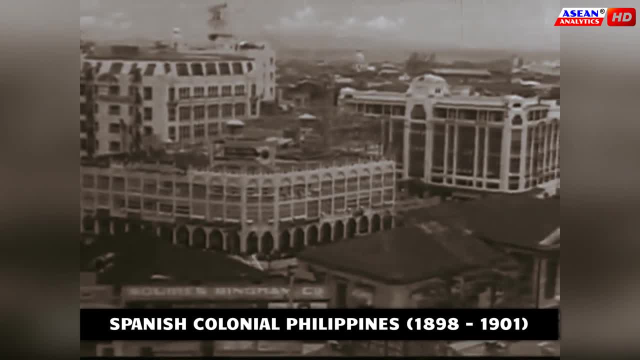 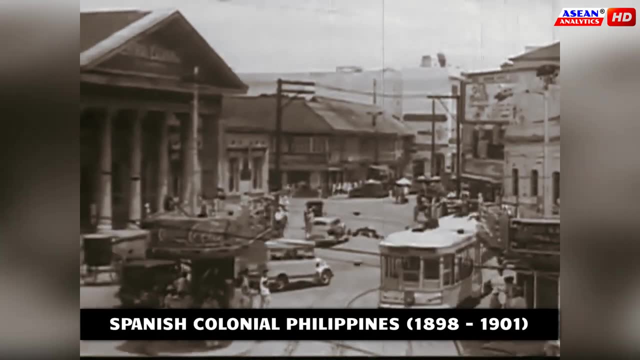 first bank opened in the Philippines and in Southeast Asia in 1851.. When the Philippines declared independence from Spain, the country was one of the most advanced economies in the whole of Asia, next only to Japan. When GDP per capita was measured in 1900, the Philippines ranked second, with GDP per capita of $1,003.. 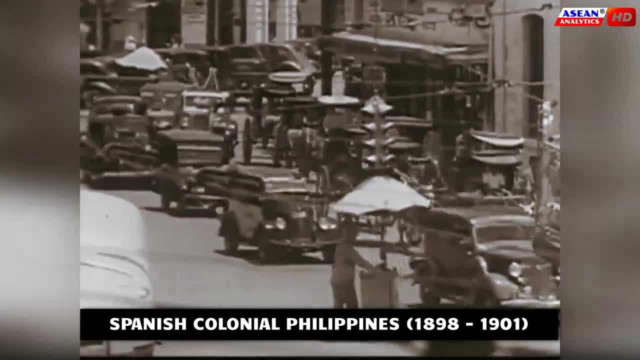 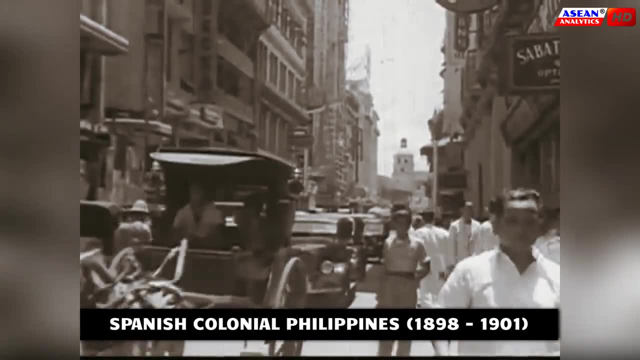 When GDP per capita was measured in 1900, the Philippines ranked second, with GDP per capita of $1,003.. it the second richest place in all of asia, just a little behind to japan with 1135 dollars and far ahead of china with 652 dollars or india with gdp per capita of 625 dollars. 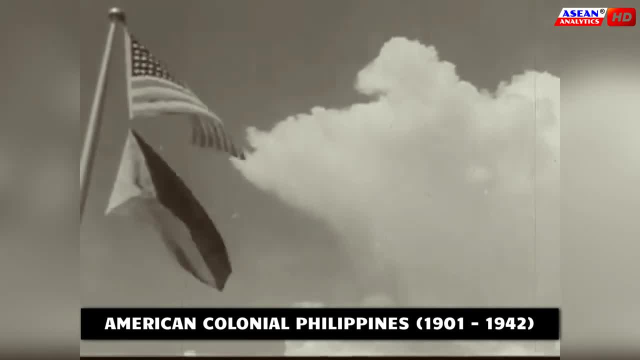 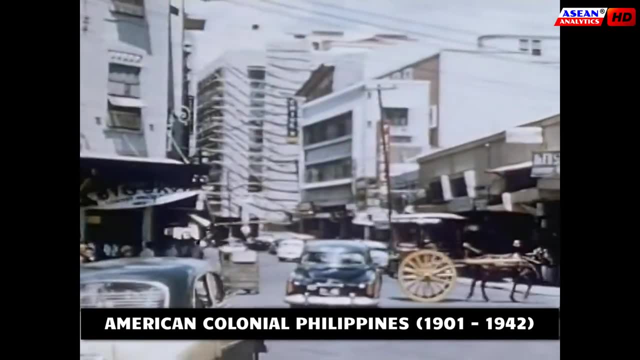 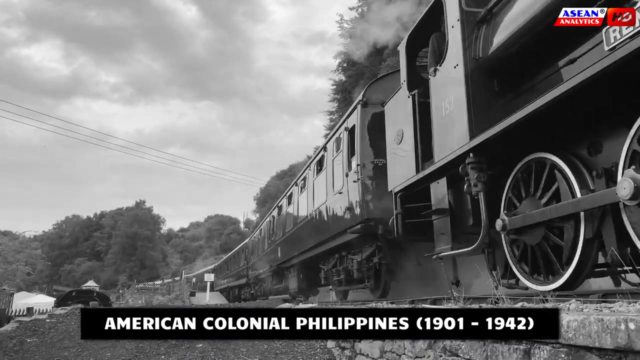 during the american colonization of more than four decades of administration, the philippines experienced a long period of relatively uninterrupted economic growth and social development. around the beginning of the american pacification of the country, there were 196 kilometers of railroads in place. by 1938 it reaches 1 353 kilometers at its peak. 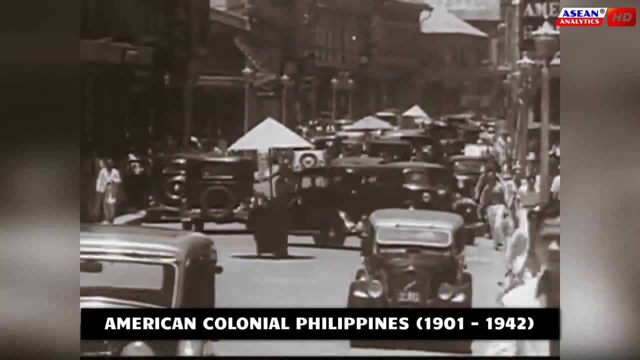 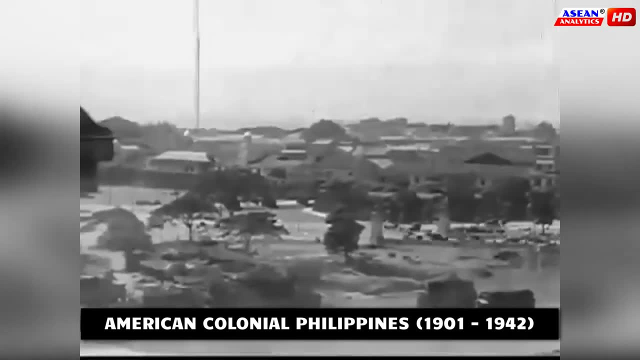 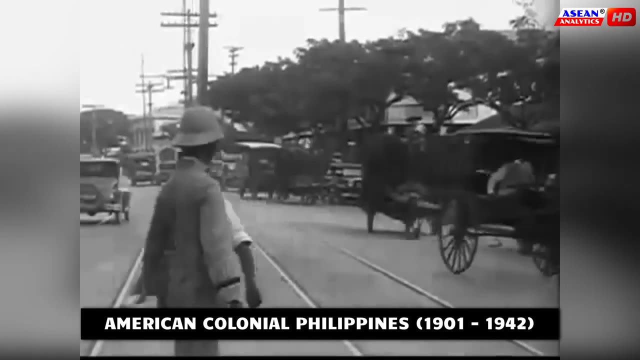 motor vehicles increased to 40 656 by 1933. roads and bridges, which were 397 kilometers in 1908, reached 15 214 by 1933.. telegraphy lines, which were five thousand 478 kilometers in 1903, had grown to 14 366 kilometers. 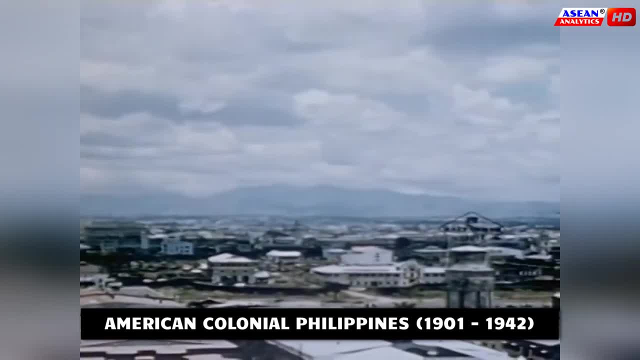 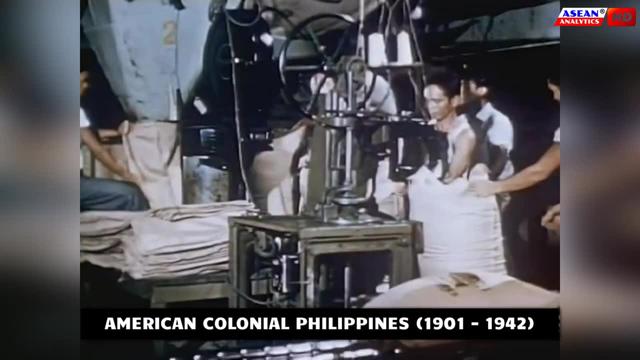 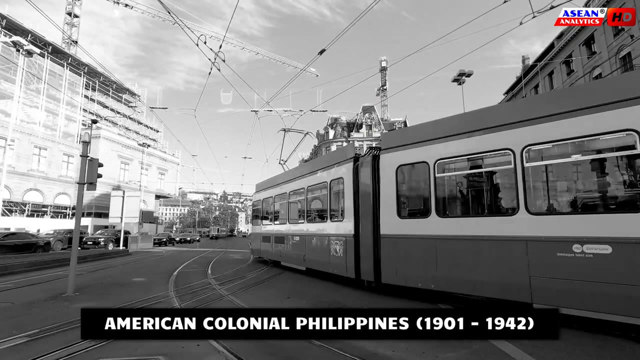 as soon as american political power was established in the country, business opportunities opened for american capital. the philippine economy became part of the larger american market. such integration enlarged its potential for investment opportunities. investments in construction, local transport and utilities were expanded as the trading relationships enlarged. 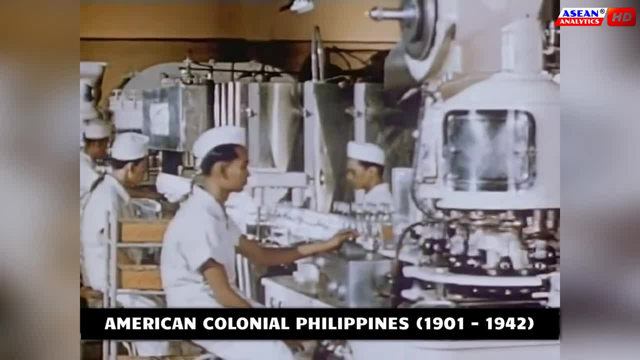 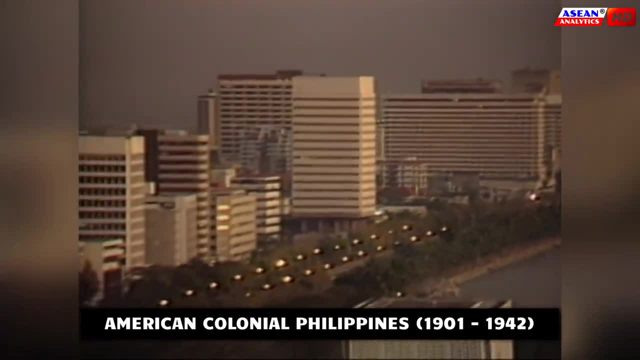 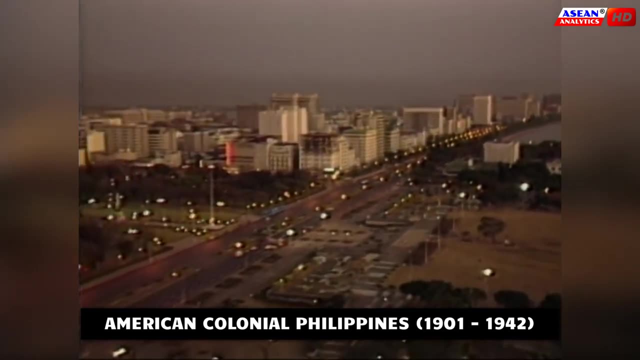 threatened american interests succeeded in getting their government to impose quantitative quotas and other forms of trade controls that would limit the expansion of philippine exports. these issues constituted sharp economic divides by the time of the clamor for independence for the colony. nevertheless, in 1940 the country was well on the way to a prosperous future. 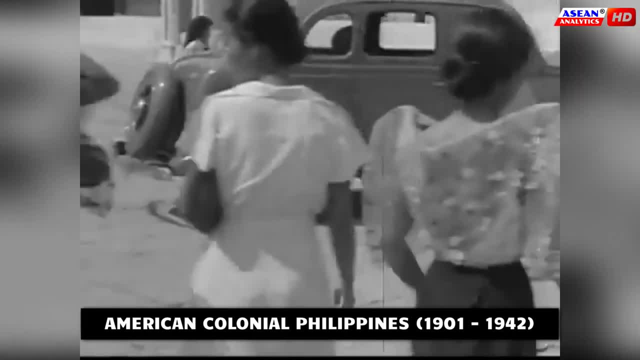 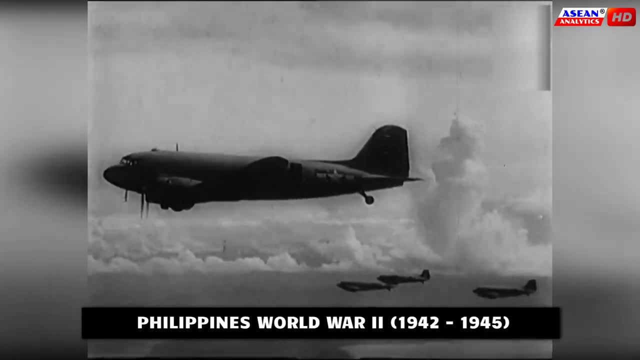 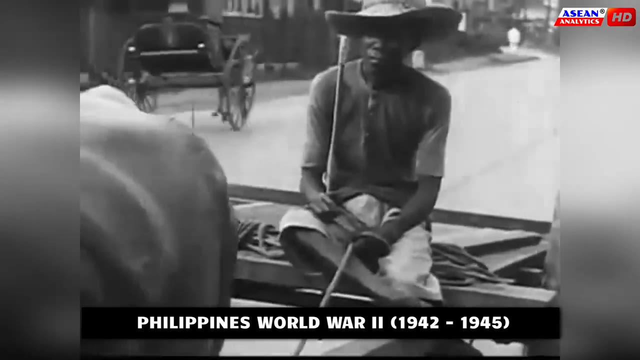 political independence was in the near future. the standard of living of the common filipino was higher in any part of southeast asia. japanese invasion during world war ii. economic growth receded and food shortages occurred. the overall condition of the economy was inexorably taking place, with production of. 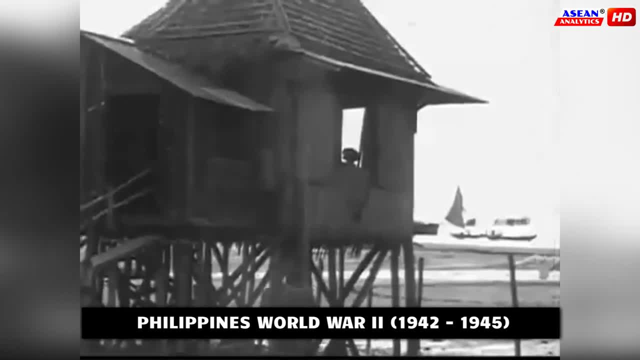 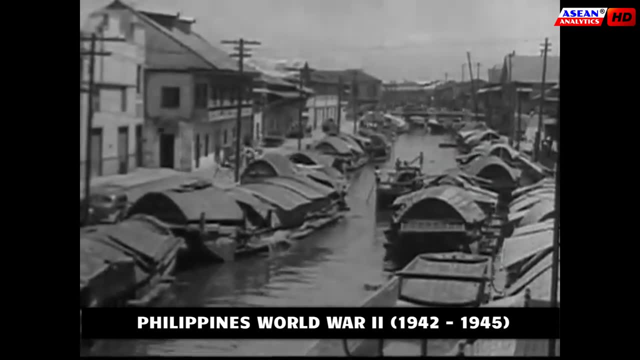 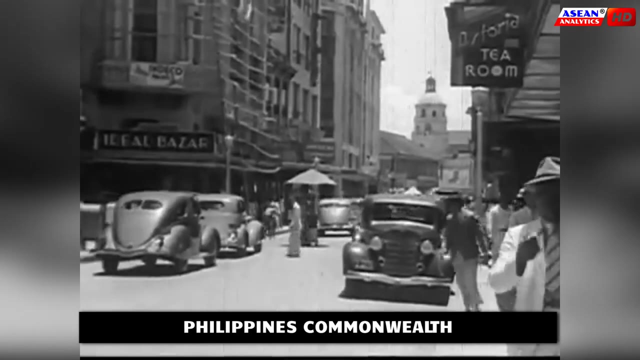 food and other products falling precipitously and supplies becoming scarce. the country also experienced the worst inflation in its history. the total output of the economy in 1945, by the war's end, was reduced to 30 of the pre-war gdp level in 1940, growth immediately after the war. 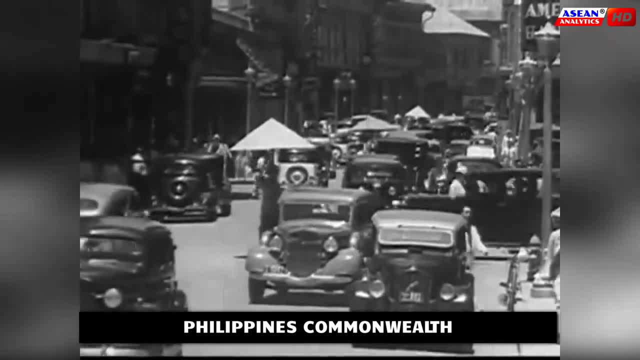 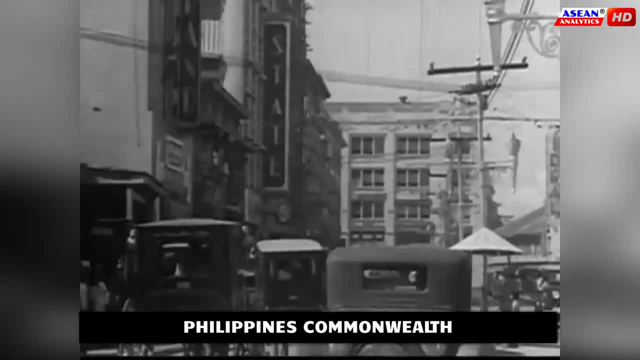 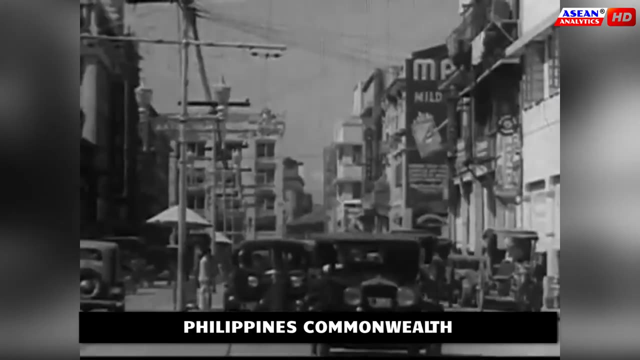 this time, the philippines become fully independent from the united states. in an effort to solve the massive socioeconomic problems of the period brought about by the war, the newly established government strengthened its finances through the revision of taxation and established international diplomacy and relations to enhance foreign trade. from the 1950s to the 1970s, the philippines was the biggest economy in all of southeast 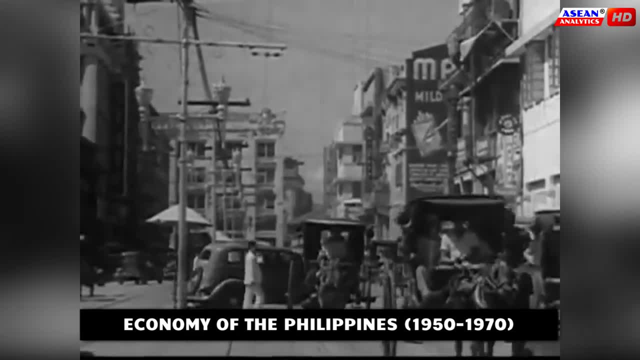 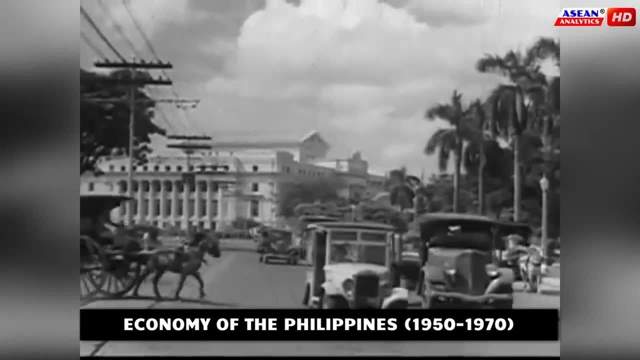 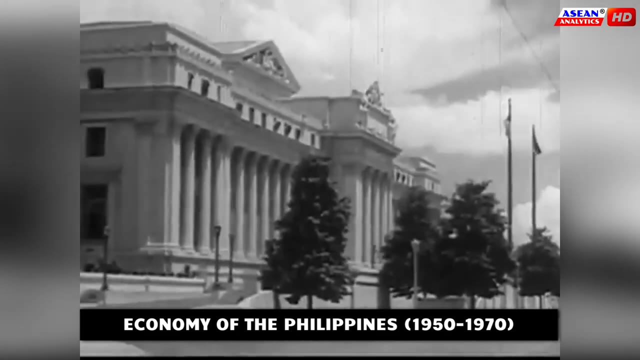 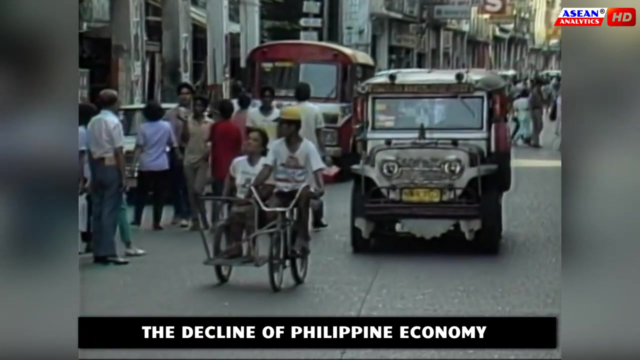 asia. despite of its smaller land area compared to indonesia, malaysia and thailand, it also, of course, maintained the highest gdp per capita in the region. the philippines economy grew at a relatively high average annual rate of 6.4 percent during this period. in the early 1970s, the currency floated as a result of the government's deficit of more than 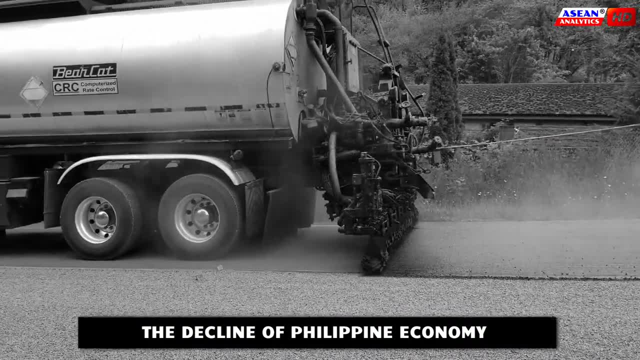 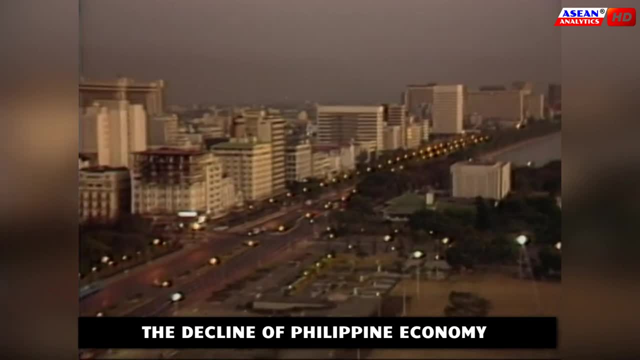 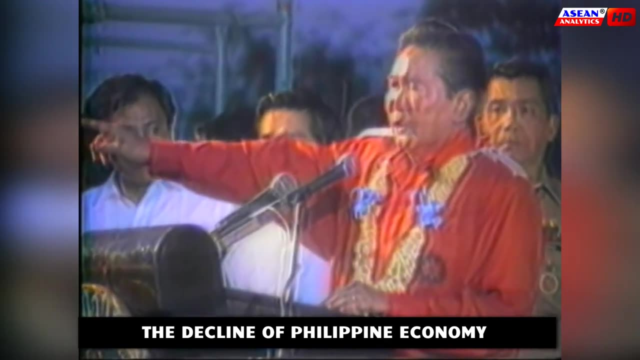 1 billion pesos as public spending was funded by public debt. the international monetary fund and the world bank underscored the modest growth of the country, despite borrowing vast money. the public debt rose to 25 billion dollars in 1983.. the declaration of martial law in 1972. 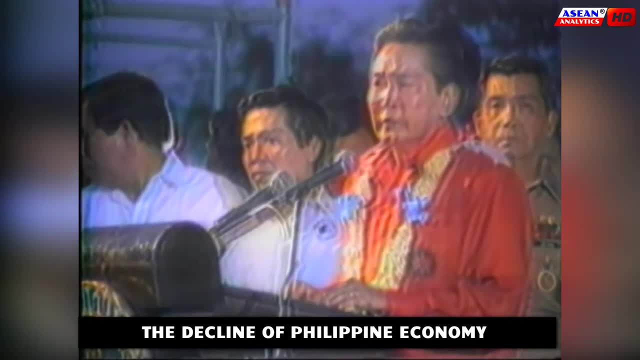 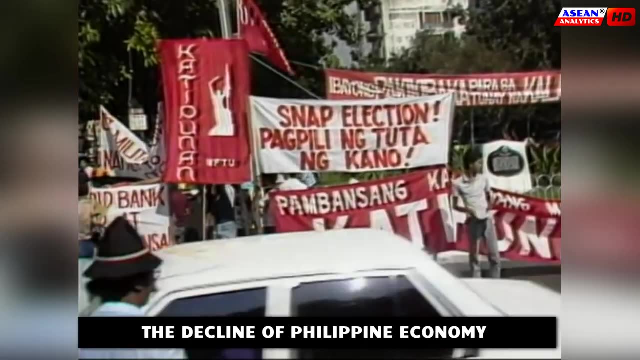 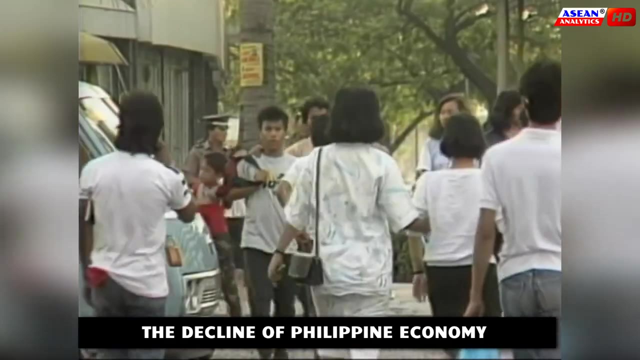 created many new opportunities for reform, but facilitated the capture of the state by newly centralized regime interests. in the 1980s, the philippine economy was hurt by political instability, authoritarianism, increasing foreign debt, falling commodity prices, corporate mismanagement and vast unemployment. the philippine economy began to run into difficulty because of 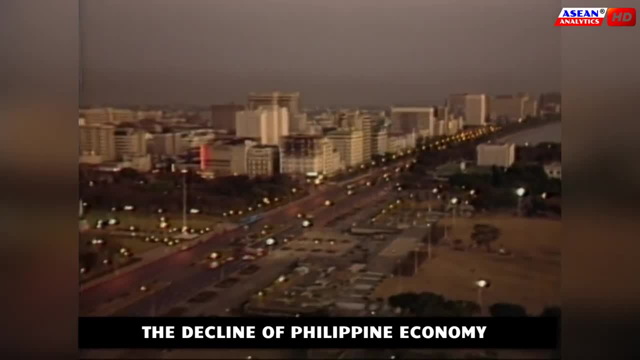 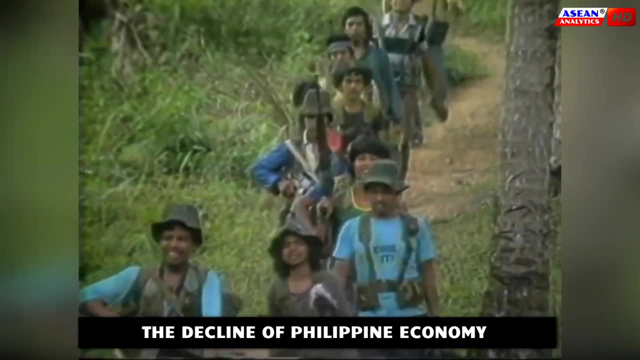 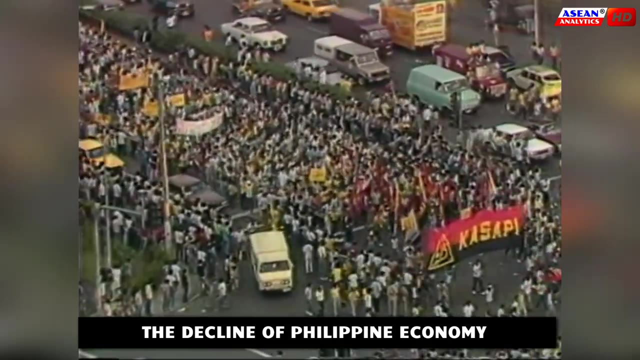 the declining world market for philippine exports, trouble in borrowing on the international capital market and a domestic financial scandal. the problem was compounded by political insurgencies. in 1983, the country descended into a political and economic crisis in the aftermath of the assassination of former senator beningo aquino, and circumstances had not improved when marcos 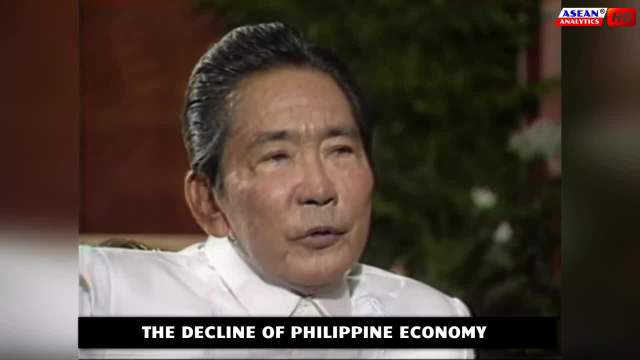 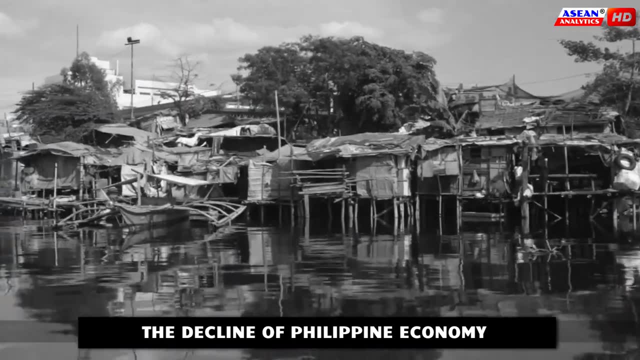 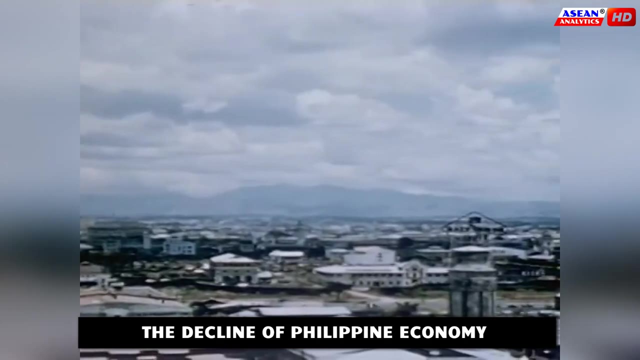 fled the country in february 1986.. the philippines was once a model for its economic development. after the fall of the philippines, the philippines became the major economic exporter of foreign goods, and they were the leading exporter of foreign goods to the east asian economies, ended up being dubbed as the sick man of asia, whose economy was driven by debt. 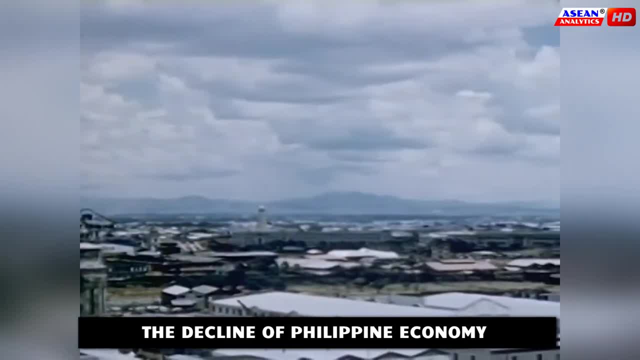 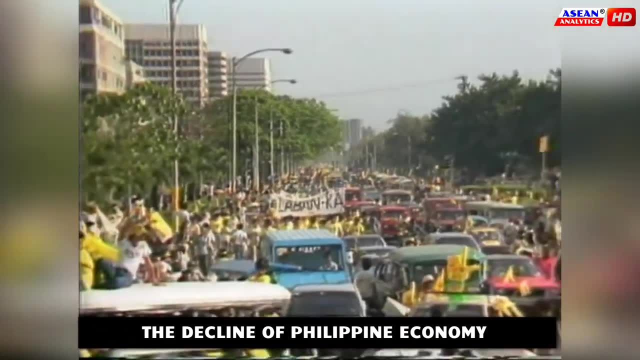 at this time the philippines has dramatically surpassed by indonesia in the early 70s, by thailand in the 80s and by the 1990s the philippines was also been surpassed by malaysia and singapore. the philippines economic recovery from the political instability in the 1980s was very slow. 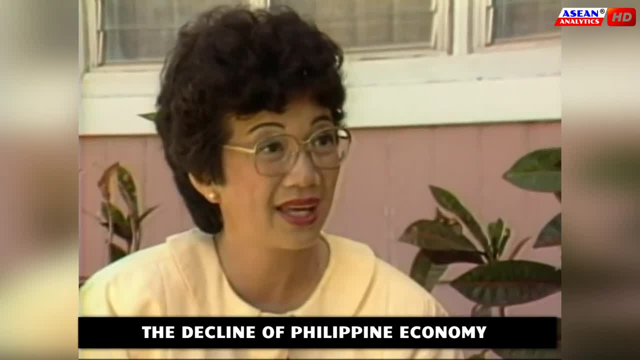 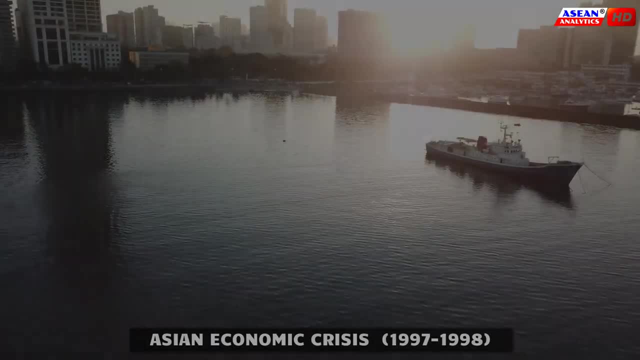 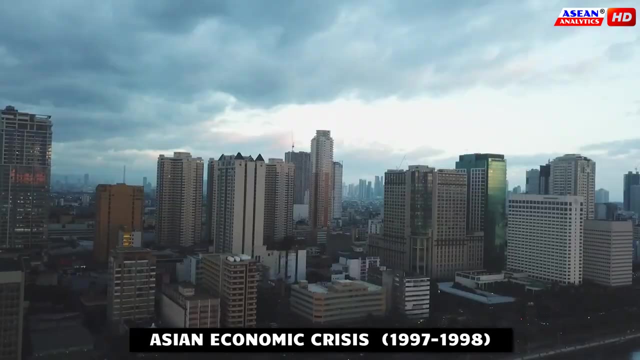 changes. Only the government type has changed, but failed to address issues thrown during the regime, like corruption, human right violation, poverty and inequality. During the Asian economic crisis from 1997 to 98, the Philippine stock market declined by 32 percent and the currency. against the dollar, depreciated by as much as 48 percent. Because many of its exports went to Europe, its economy was not hurt that badly. Money sent home by Filipino workers abroad helped stabilize the currency. Even so, the Philippines recovered more slowly after the crisis than some. 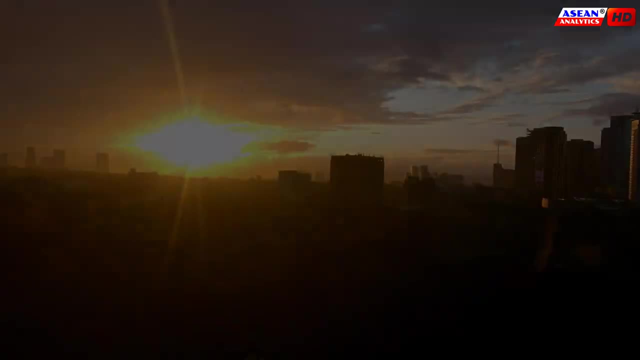 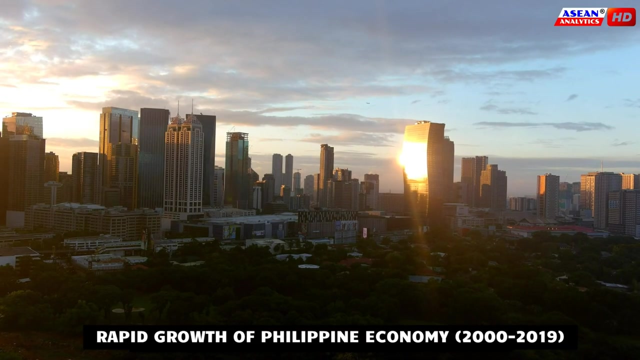 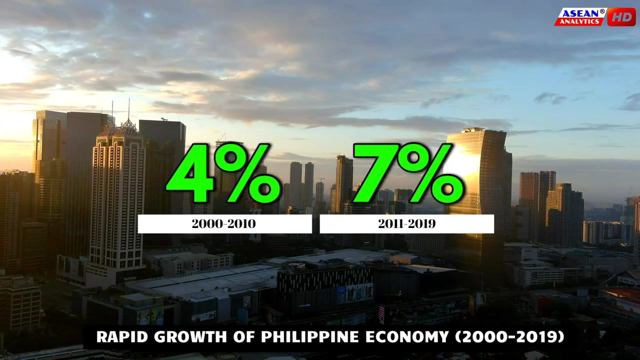 other Asian countries that were much harder hit. The gloomy days of the Philippines economy start fading in the early 2010s. Philippine economy picks up and its average growth rate from four percent significantly rises to seven percent, surpassing its neighboring country in the 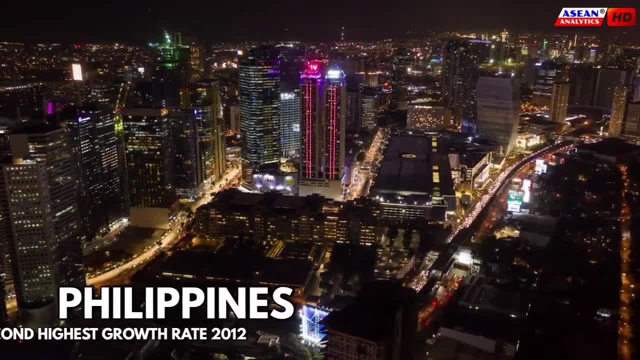 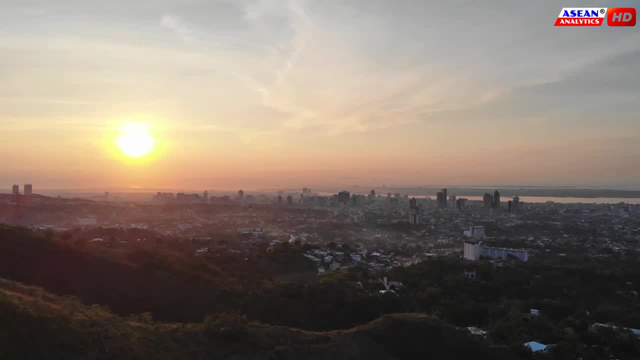 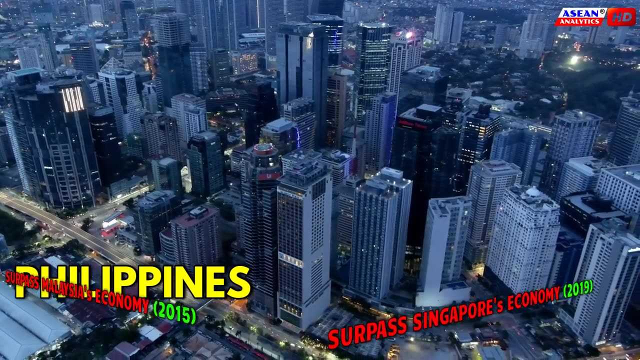 region. The Philippines had the second highest growth rate in the world in 2012, after China. This is the comeback of the country's stable economy In 2015,. the Philippines surpasses Malaysia in terms of economic size and in 2019, regained its spot as the third biggest economy. 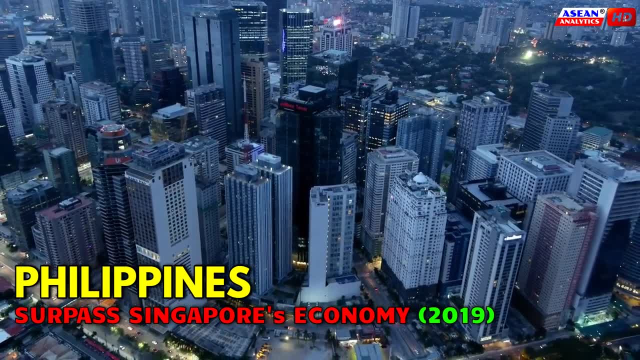 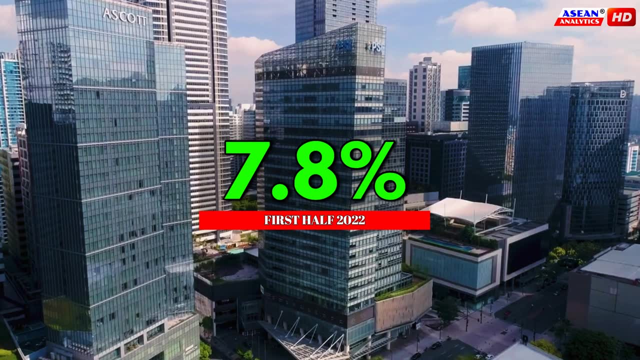 in Southeast Asia. after surpassing Singapore's nominal GDP. Currently, the Philippines is considered the strongest economy in the region after China. The Philippines' economic growth rate is 7.8 percent after the economic setback during the pandemic, with an average growth rate of 7.8 percent. The country also intensively modernized and expand its public infrastructure to enhance mobility and spurs economic development to the country. In the past six years of rebuilding the country, the Philippines' infrastructure significantly improved, especially in the sector of aviation, railways, bridges, urban development and roads and expressways.